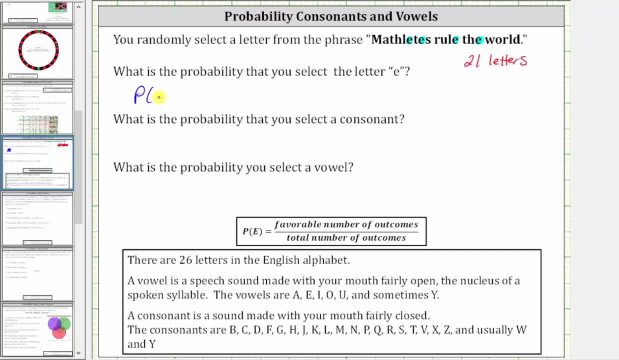 and therefore the probability of selecting an E- we'll call it probability of E- is equal to four divided by 21,. again, because 21 is the total number of outcomes. This fraction doesn't simplify, so this is the exact probability, but let's also show that 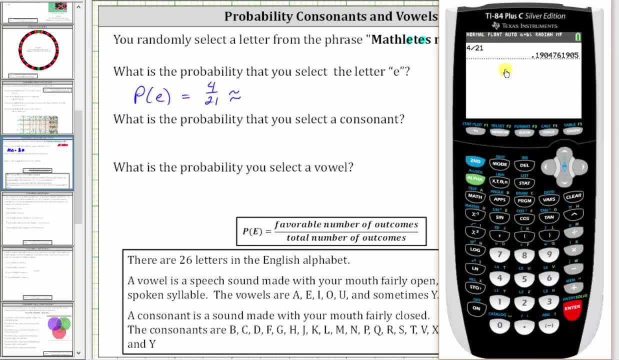 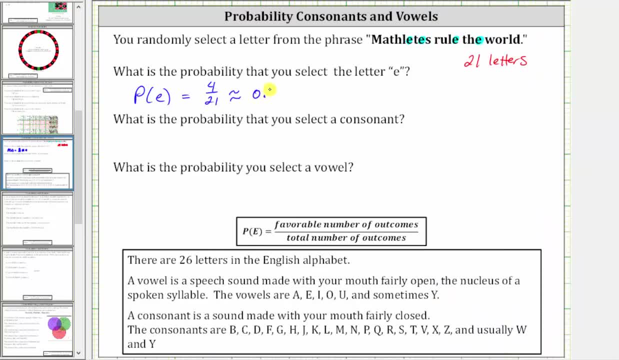 the probability is a decimal and a percent. If we round to four decimal places, four divided by 21 is equal to 0.1905, which is equal to 19.05%. Next, we're asked to determine the probability. you select a consonant. 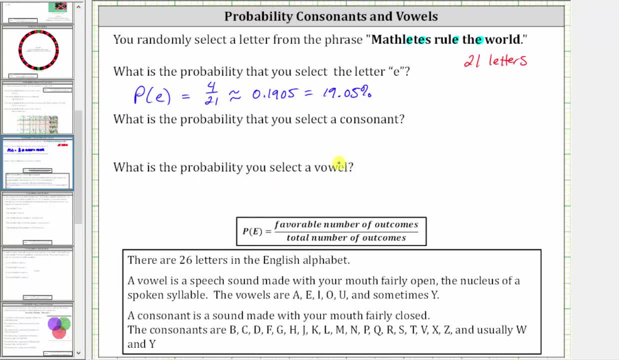 and then the probability. you select a vowel. Look in our notes below The vowels are A, E, I, O and U, and sometimes Y, but we'll assume they're just A E, I, O and U. 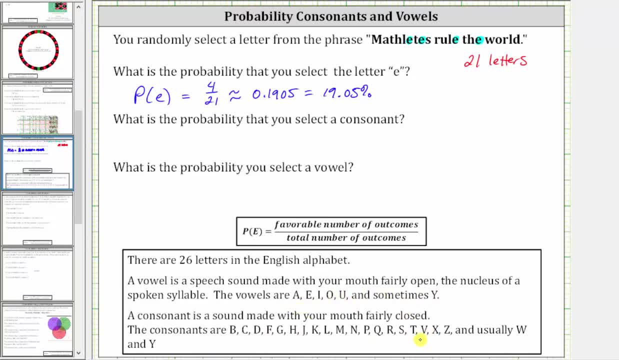 And the consonants are the letters that are not vowels, listed here. So let's find the probability. you select one letter and it's a consonant. Actually, it might be easier to count the vowels first, which will also help us with number three. 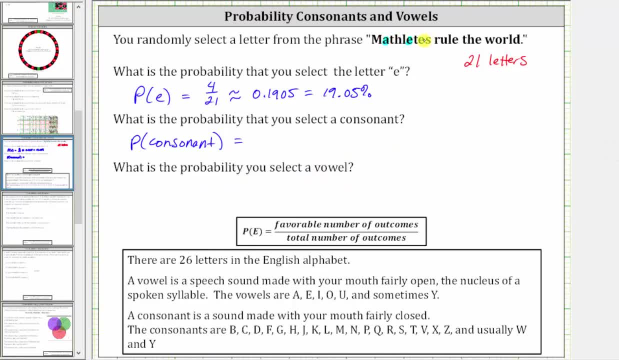 So the vowels are A- E. there's another E, U and E, E and O. So there are one, two, three, four, five, six, seven vowels. Let's make a note of that: seven vowels. Well, if there are 21 letters and seven vowels, 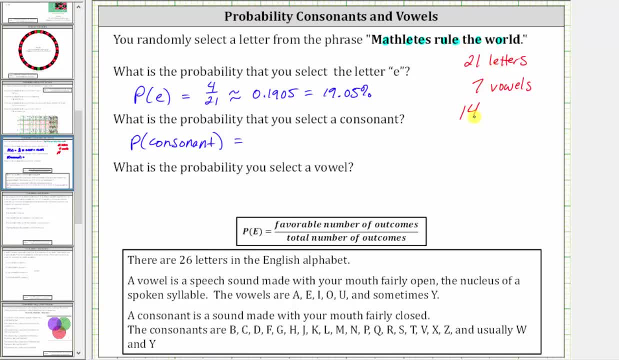 21 minus seven is 14, there must be 14 consonants. Of course, we can count them, which does give us 14 consonants. So the probability you select a consonant is 14 divided by 21 or 14 21sts, which does simplify. 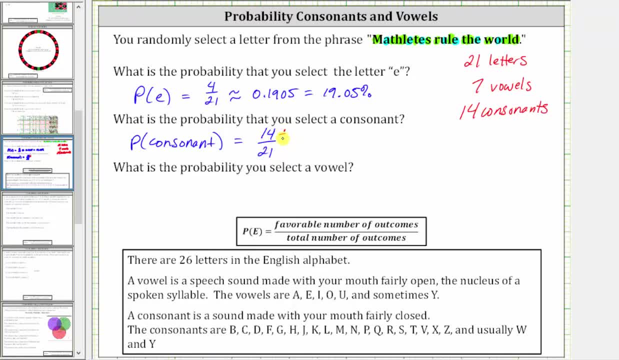 14 and 21 share a common factor of seven. Simplifying you divide both by seven, which gives us two thirds, which we should recognize as a decimal, is 0.6 repeating. So if we round to four decimal places, this is approximately 0.6667,.